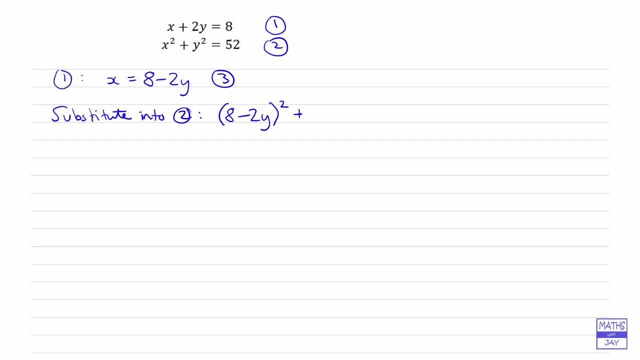 And then we just write down the rest of equation 2 as it was, so that you can see that all we've done is replace x by 8 minus 2y, and now we've just got an equation in y, so we need to multiply out the 8 minus 2y squared. so that's the same. 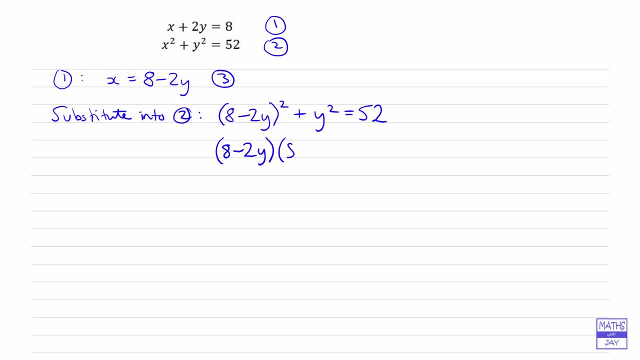 as 8 minus 2y multiplied by itself and everything else. whoops, we don't want that squared there and everything else stays exactly as it was in the previous line. so we've just written 8 minus 2y times 8 minus 2y instead of 8 minus 2y, squared right. so. 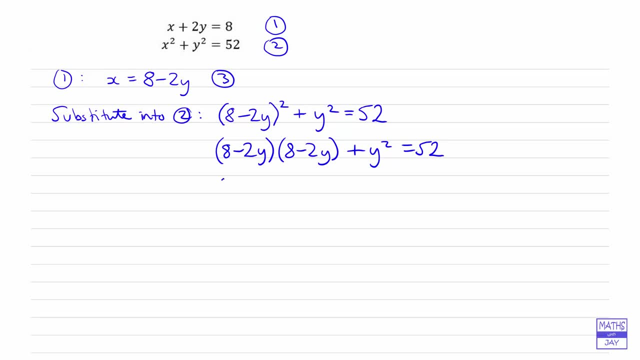 let's multiply out those brackets: 8, 8s are 64, and then we've got 8 times negative 2y and that we've got that twice, so it's two lots of minus 2y squared. So that's minus 16y, so it's minus 32y and then negative 2y all squared is going to be. 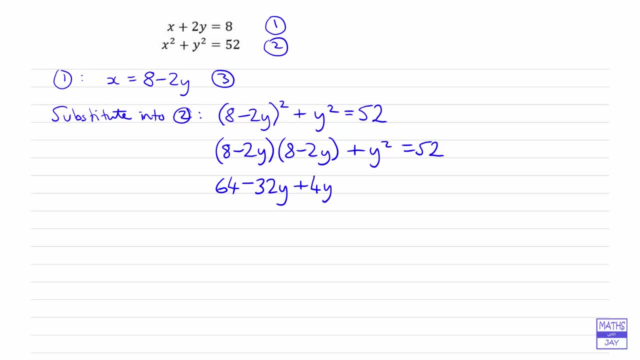 plus 4y squared, because a negative multiplied by negative is a positive, and then, as before, we've still got the plus y squared equals 52.. So what we're aiming to do here is to write this as something times y squared plus something times y plus a constant. 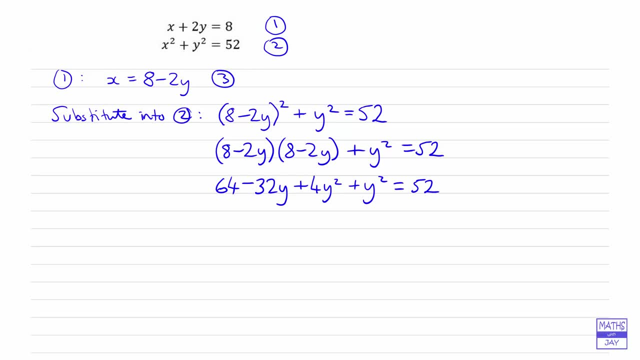 Equals zero. and then we're hoping to be able to factorise the quadratic. So 4y squared plus y squared is 5y squared. And then we're taking away 32y, and then we've got plus 64, but on the other side we've 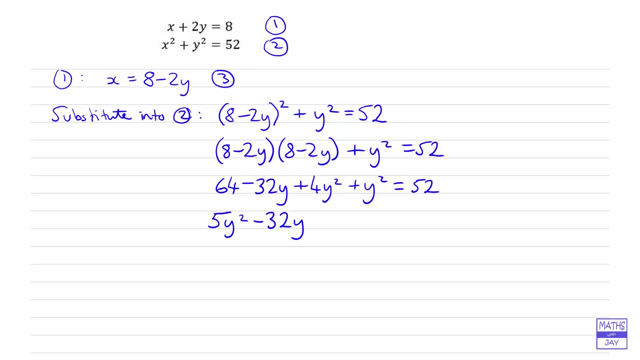 got 52, so we're going to take 52 away from both sides, so that will give us plus 12 and equals 0.. So we can now factorise this and it's not too bad because we've got a prime number multiplying the y squared, so we must have 5y and y. 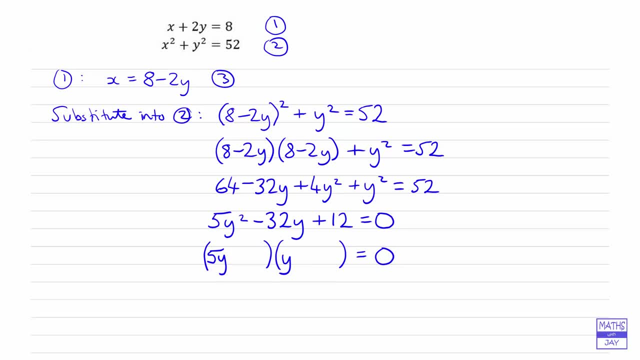 We have got plus in front of the constant, but minus in front of the other term, in front of the 32y, so we know we must have a minus and a minus. The next part's a bit tricky because we know that 12 can be written as 1 times 12.. 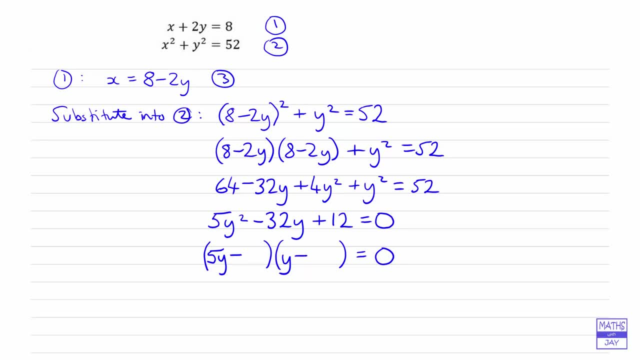 2 times 6 and 3 times 4.. So we need to think a little bit about what numbers we're going to be putting in here. So it can't be 1 and 12, trying out some different possibilities, but we can see that it is going. 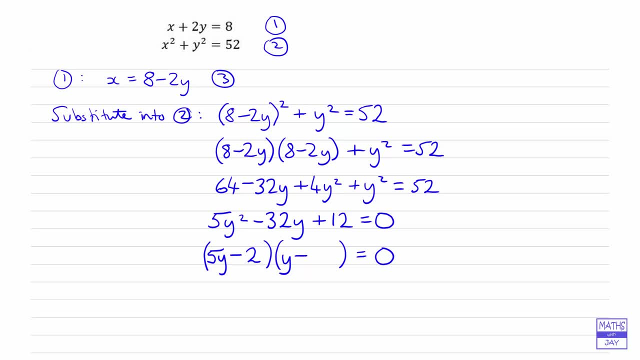 to be 2 in there and 6 in there, because minus 2y and minus 6 times 5y comes to minus 32y. And then this will give us our two solutions: 5y minus 32y, Y minus 2 is 0 or y minus 6 is 0. 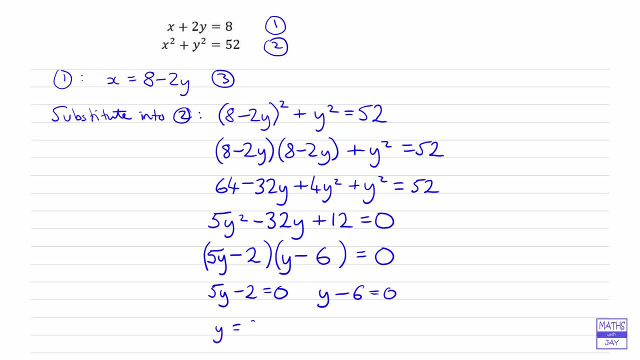 So y is either going to be 2 fifths or 0.4, or it's going to be equal to 6.. So that's the hard work done. but we need to remember we've got to find x as well, So let's just reduce this down in size. 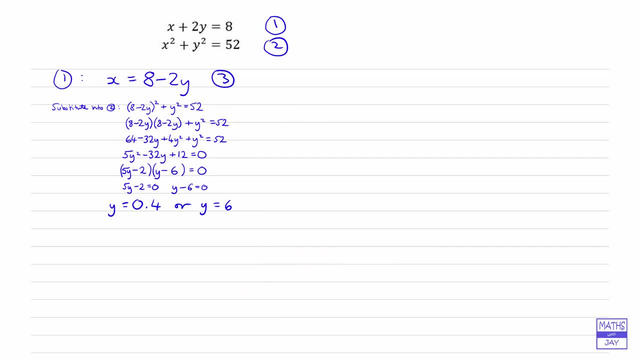 So now we've got to find the value of x. We know the value of y, So the best equation to use now is equation 3, because that gives us x in terms of y. So let's start with: y is 0.4.. 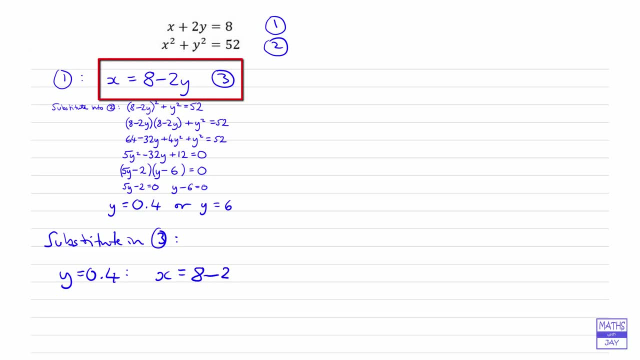 And so the equation 3 gives us that x is 8 minus 2 times 0.4.. So that's 8 minus 0.8.. So that's 7.2.. And it's a good idea to check your answers as you go along. 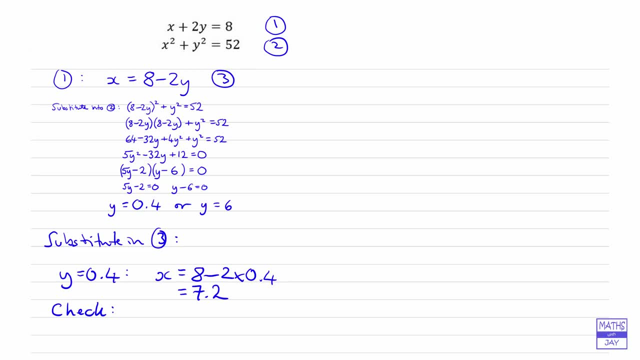 So we've effectively used the linear equation here, haven't we at the end? So now let's check in equation 2.. So we want to find out what x squared plus y squared is equal to, And that's going to be 7.2 squared plus 0.4 squared. 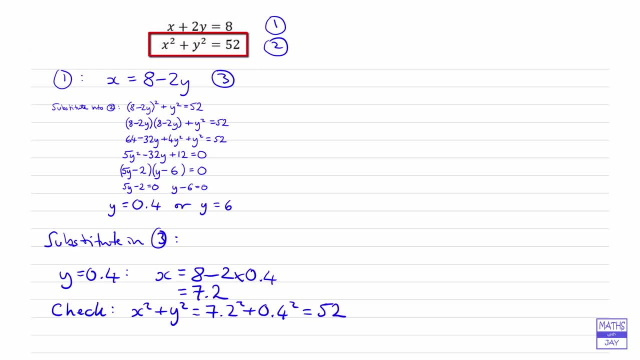 And that does indeed come to 52.. So that's a good start. And then we've got to find the value of x, So that's 7.2 squared plus 0.4 squared, And that does indeed come to 52..